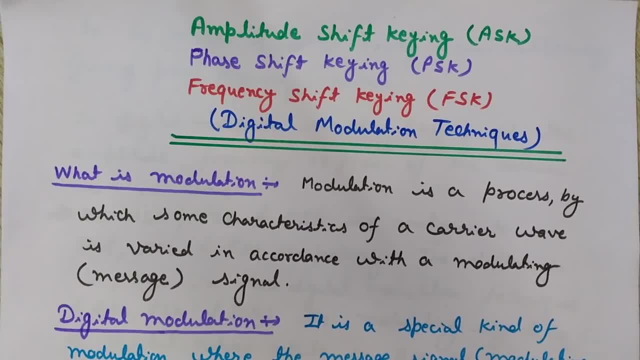 in accordance with a modulating, also known as messenger baseband signal. So what we do in modulation? we have a high frequency carrier wave and we change the either frequency, phase or amplitude of this carrier wave according to the variations- instantaneous variations- of the 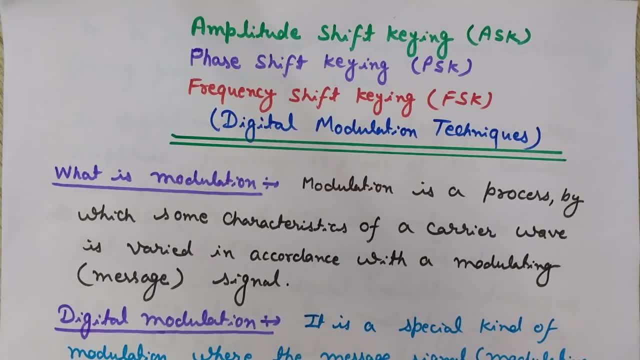 message signal. So if the amplitude of the carrier wave is varied, then we will call it as amplitude modulation. If frequency or phase is varied of the carrier wave, then it would be known as frequency or phase modulation. So now it is time to understand what is digital modulation then. So digital modulation is a special 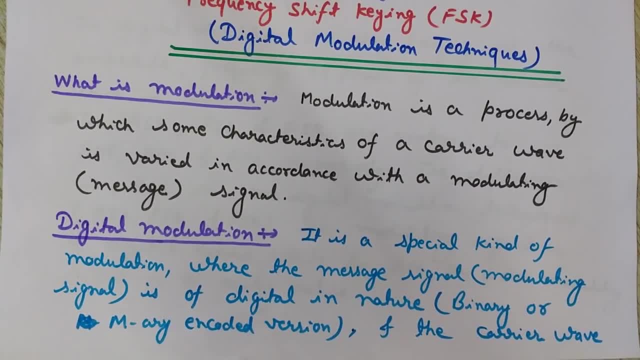 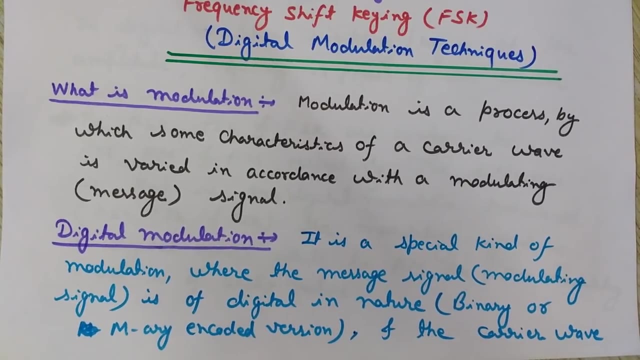 kind of modulation where the message signal is of digital nature, It may be binary or amery encoded version, And the carrier wave is of analog nature. So you can understand here that in analog kind of modulation, where its examples are AM, FM and PM, we have two. 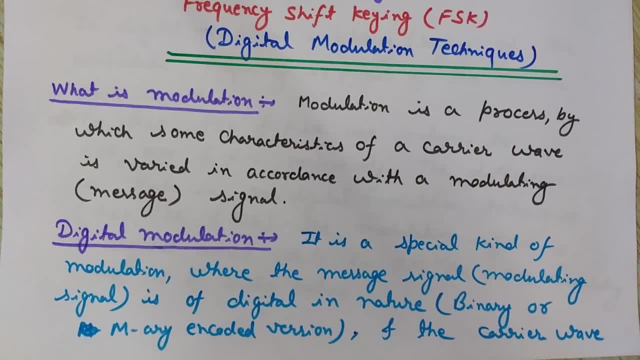 is sinusoidal carrier wave. so in this digital modulation case also we have analog carrier wave. but the difference between analog and digital modulation is based on the message signal, that is the modulating signal. in analog kind of modulation the message signal, the modulating signal, is of analog nature, but in digital modulation, thus this modulating signal is: 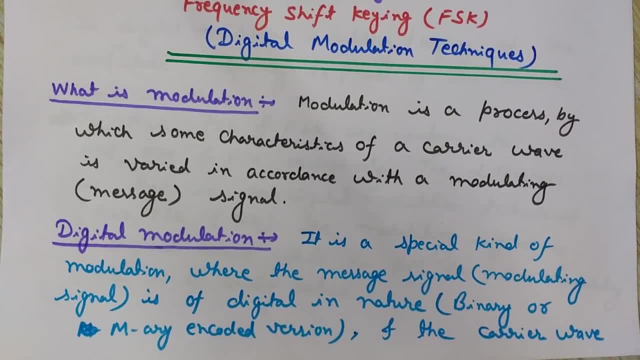 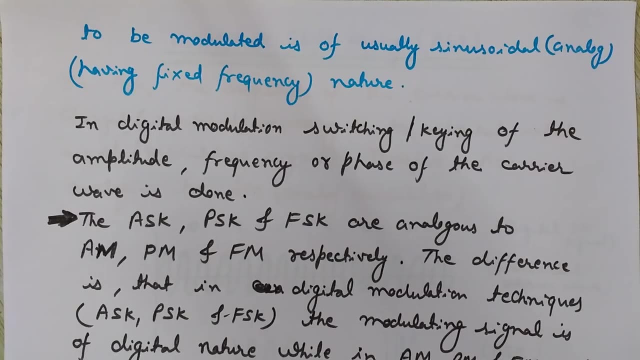 of digital nature, so we may either use the binary or mra encoded version. while transmitting in in mra encoded version, instead of transmitting one bit at a time, we transmit two or more bits at a time. okay, so it reduces the bandwidth. the carrier wave used in digital modulation techniques is of 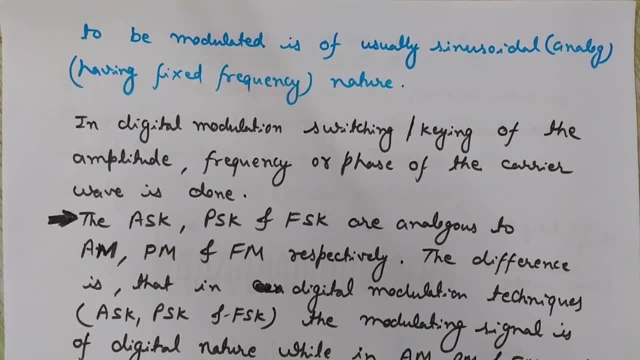 analog and generally of sinusoidal nature. okay, so what we do in ask psk and fsk? actually in digital modulation techniques, we are doingругer multiplication, two-times bigger edition. you are alsoส1 восaires the bandwidth, the carrier increase in a digital modulation stuck to the digital. 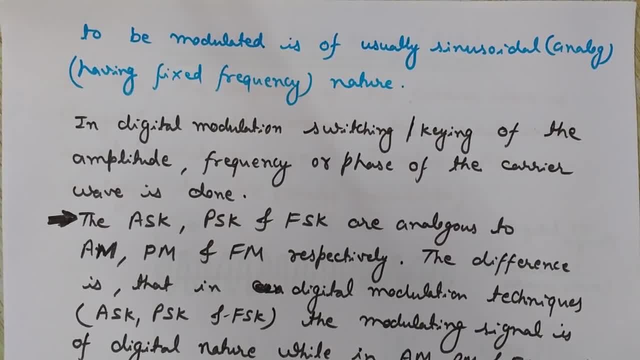 promoting circuit waiting suggest that we are giving close to each other operation of the homo in modulation switching. this is known as the switching or keying of the amplitude, frequency or phase of the carrier wave. okay, as per the message signal, the ASK, PSK and FSK are analogous. 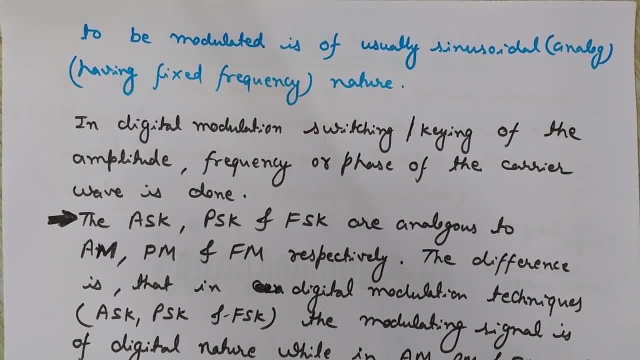 to AM, PM and FM respectively. as I have already told you that the difference is that in digital modulation techniques, the modulating signal is digital in nature, while in analog modulation techniques like AM, FM and PM, the modulating signal is of analog nature. okay, so this is. 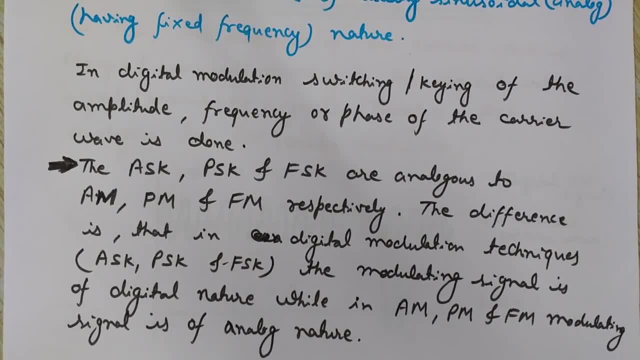 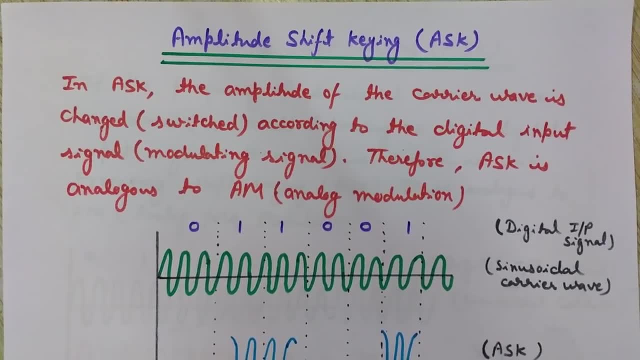 written here. okay, so now we will discuss ASK, FSK and PSK in detail separately. okay, so let's start. so first of all, we will see the amplitude shift keying ASK. in short, in ASK, the amplitude of the carrier wave, which is of analog nature, is changed. or we say: 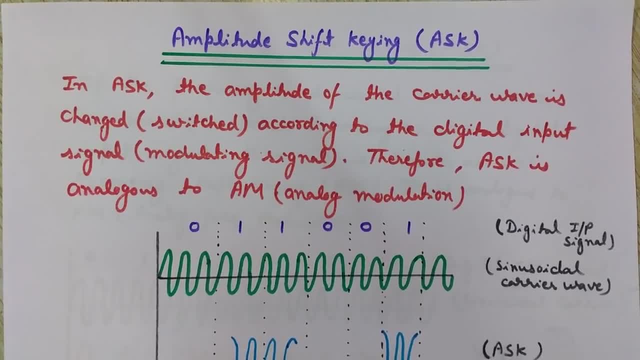 you. it is switched according to the digital input signal, since we know that the modulating signal here is of digital nature. therefore ASK is analogous to AM. AM is a kind of analog modulation because in amplitude modulation also we changed the. we vary the amplitude of the carrier wave. 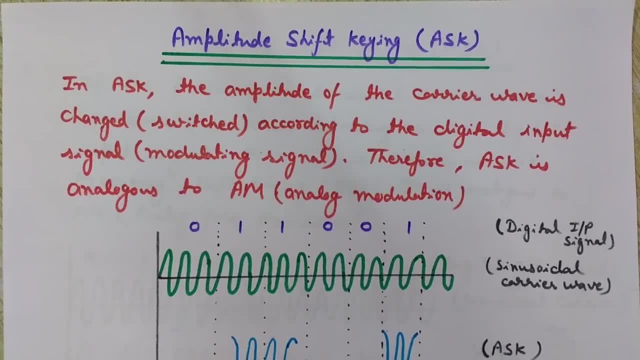 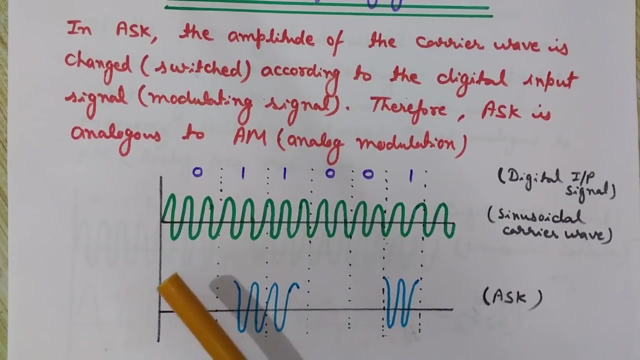 according to the instantaneous value of the message signal. so here also the difference is only of message signals nature, where it is. here it is digital in nature. so here we switch the amplitude of the carrier wave according to the digital input signal. let's understand it with this example, very simple and interesting example. so here: 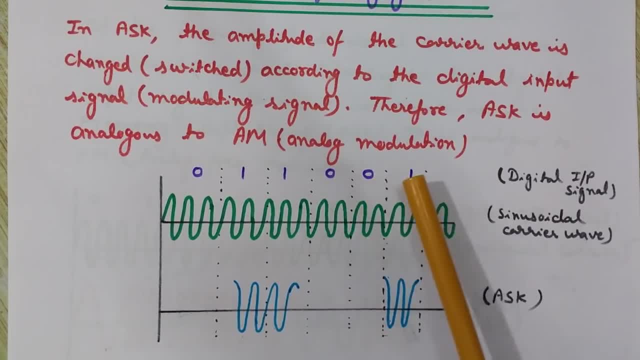 this is 01 10001. this is digital input signal. this is the digital input signal. as I told you, the message signal or the or the modulating signal is of digital nature. so this is binary digital nature and this is the carrier wave. we know that the carrier wave is sinusoidal, that 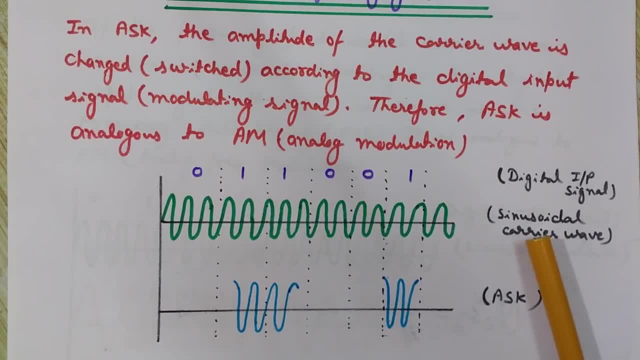 is analog in nature, like the analog modulation. so here also, the modulating signal is digital and the carrier wave is analog. now we wanted to change the amplitude of this carrier wave according to this binary sequence, according to this digital binary signal. so what will we do here? 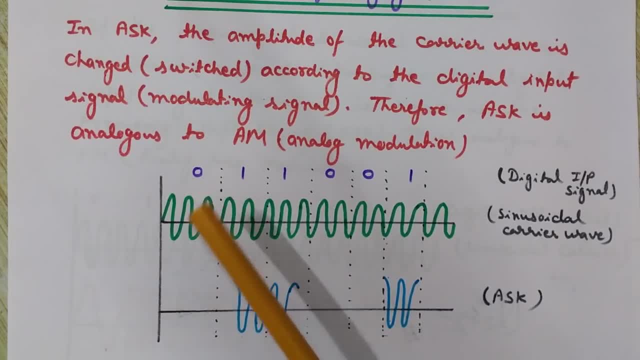 in amplitude shift keying, we do not transmit any signal. when it is zero, okay, and when it is one, then this carrier wave is transmitted. so as you can see here that at the places where it is zero, zero, zero and zero at three places, it is clear from this example that at these three 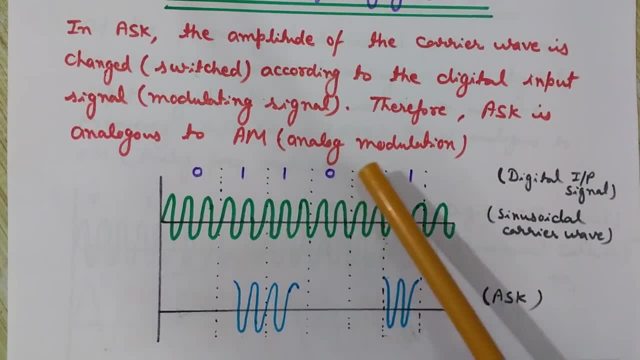 places one, two and three where it is zero. at these three places, no signal is transmitted, no carrier wave is transmitted. it is zero, okay, nothing is transmitted. and at the places where it is one- at this, this and this place- we transmit continuous carrier wave. so here and here we have 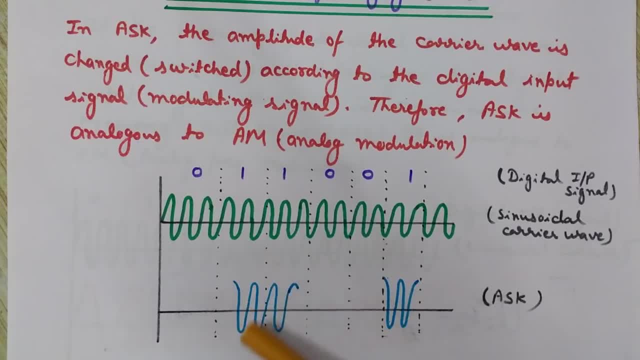 two ones, so continuous wave, the continuous carrier wave, sinusoidal wave is transmitted. if we had a three continuous ones here, then we will allow this carrier wave to trans, to be transmitted till these three ones. so it is very clear, so you can understand here that the amplitude of this 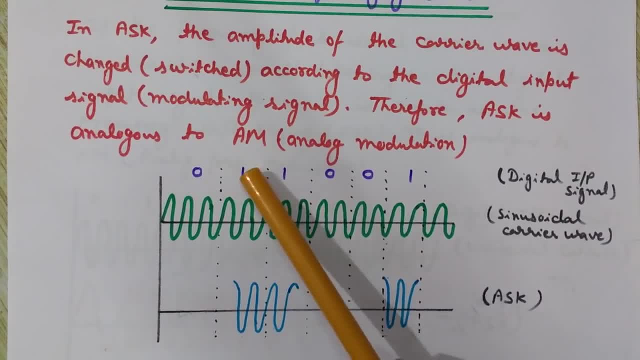 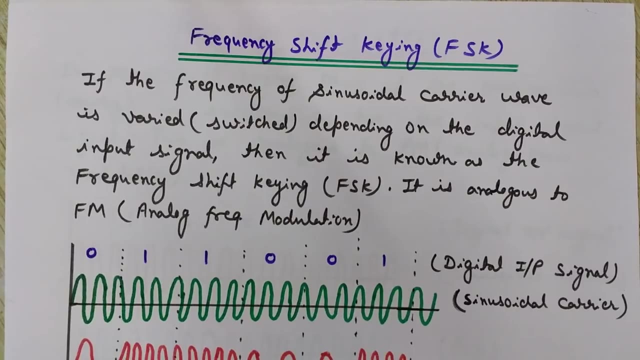 carrier wave has been changed according to this digital input signal. okay, now we will see the frequency shift keying, fsk. okay, so here is the frequency shift keying if the frequency of the sinusoidal carrier wave is varied or switched or keyed, depending on the digital input signal. 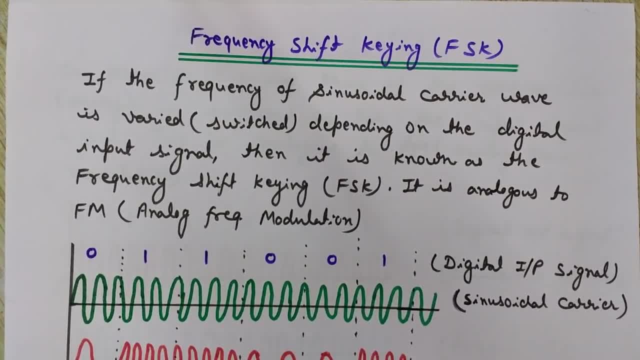 then it is known as the frequency shift keying, fsk. it is analogous to fm, which is a type of analog frequency modulation. so since in frequency modulation, which is of analog type, we just change the frequency of the carrier wave according to the instantaneous value of the carrier wave, 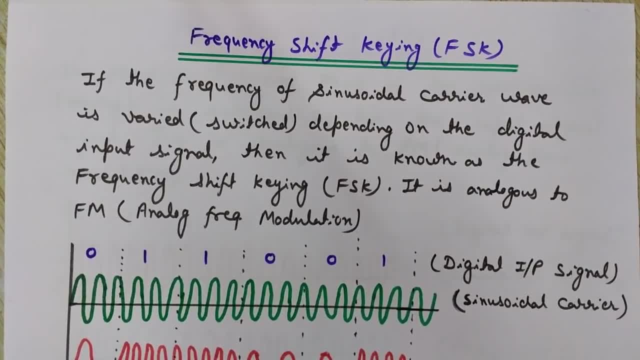 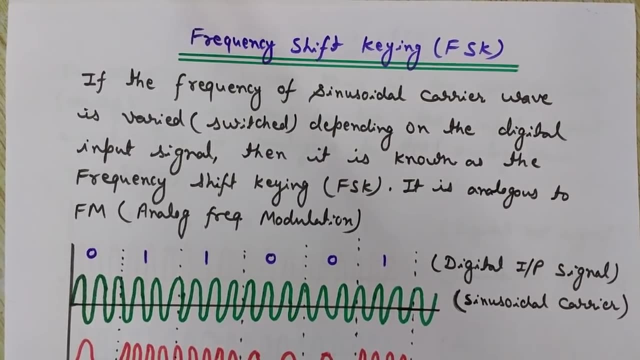 the modulating signal. okay, so in this case also, only the difference is of modulating signal which is digital in nature. so we change the frequency of the sinusoidal carrier wave or it is switched according to the digital input signal. so this is an example. so this is the concept, how this 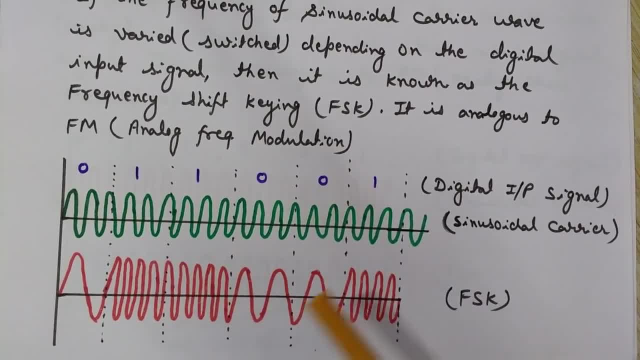 fsk takes place the process of fsk. so this is 0: 1, 1 0, 0, 1. this is the digital input signal. okay, and this is the carrier wave analog kind. this is digital, this is analog and here the we have shown the frequency shift key. so it is very easy to note here that see here, when zero is to 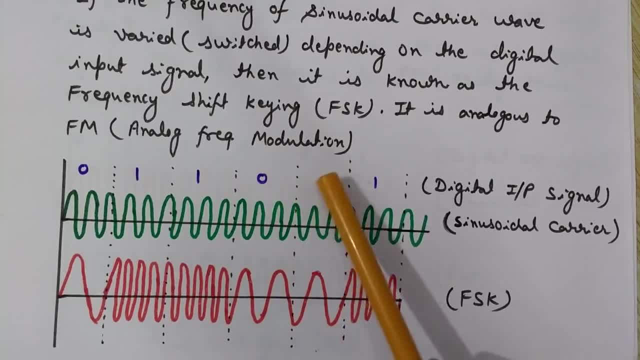 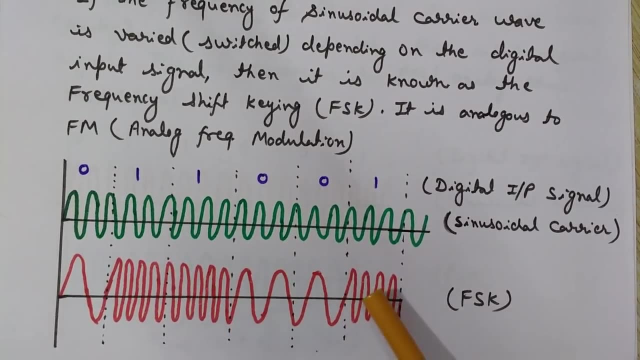 be transmitted at these three places: zero, zero and zero. you can see the wave form. okay, it is having low frequency at these three places, at this place, this place and this place, and when one is to be transmitted, we have high frequency of this carrier wave, okay. so since 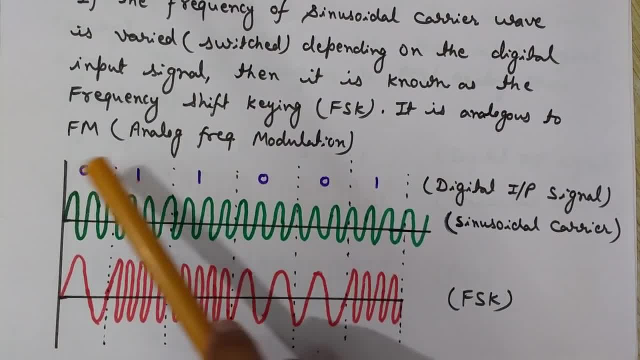 it is a frequency shift keying. therefore, as per this digital input signal that is either zero or one is transmitted, we are changing the frequency of this carrier wave according to this digital input sequence. we reduce the frequency of this carrier wave according to this digital input sequence. we reduce the frequency of this carrier wave according to this digital input sequence. we. 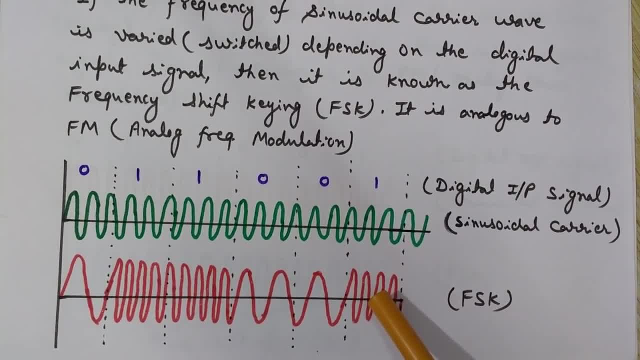 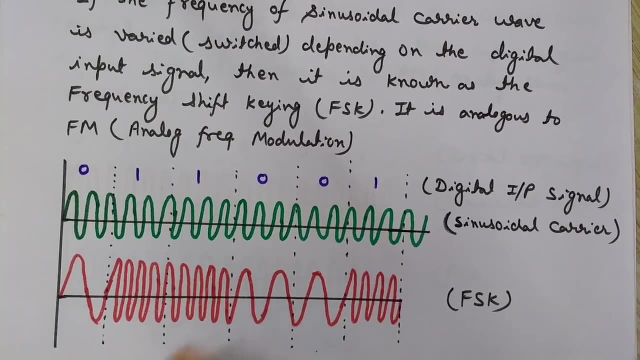 reduce the frequency when zero is transmitted and we increase the frequency when one is transmitted. okay, we know what is frequency. frequency is the number of cycles that are passed in one second. okay, so it is higher when one is transmitted and lower at zero is transmitted. now let's see the. 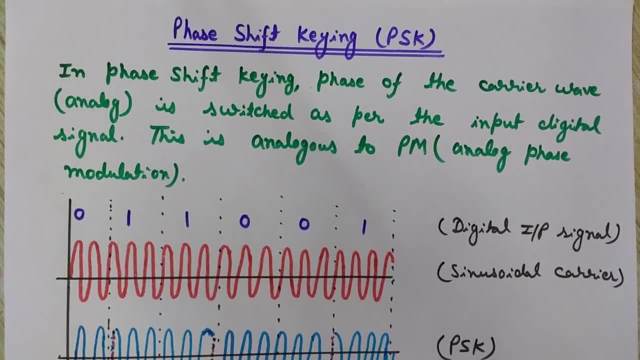 phase shift key, psk, known as the skin shot. in phase shift key we have the lower at zero, the lower is transmitted. when then we increase frequency, so as we increase frequency of the neurotransmitters, the phase of the carrier wave, which is analog, is switched as per the input digital signal. 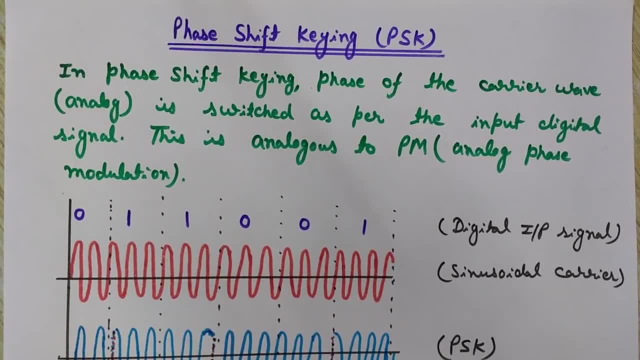 this is analogous to pm, that is, phase modulation, which is a kind of analog phase modulation. the concept is same as before. in phase modulation, analog phase modulation, the phase of the carrier wave is varied according to the instantaneous value of the message signal modulating signal. okay, so in this case also, since it is just digital kind of modulation, the sequence, the 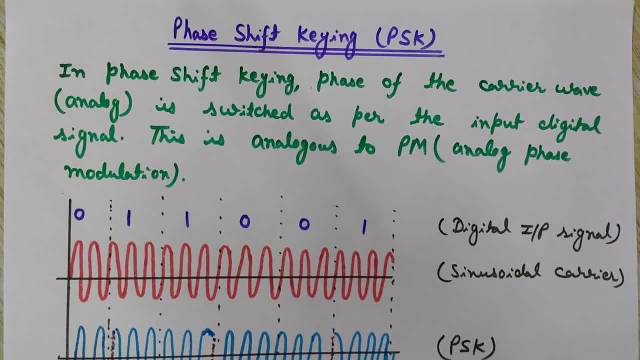 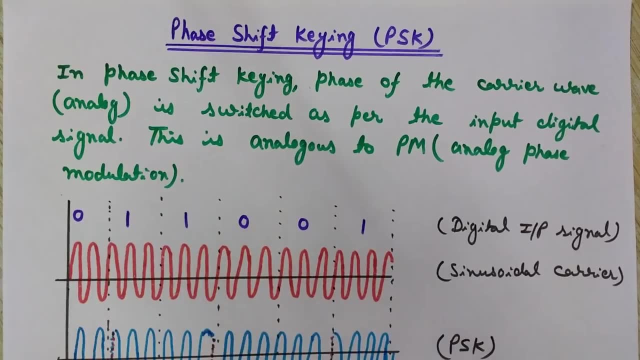 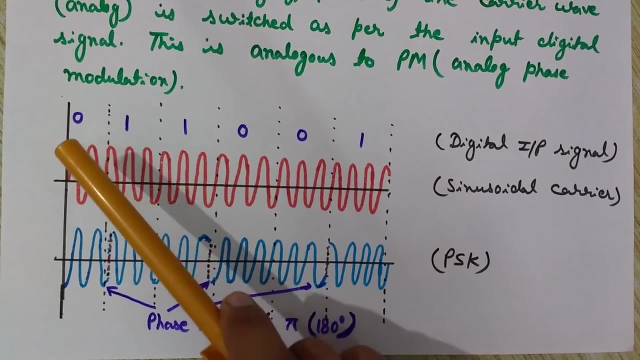 input signal is of digital nature and the carrier wave is varied or switched according to this input digital signal. so let's understand the concept with the help of this beautiful waveform. so here we have this digital input signal: 0, 1, 1, 0, 0, 1, and this is the carrier wave, analog in nature. 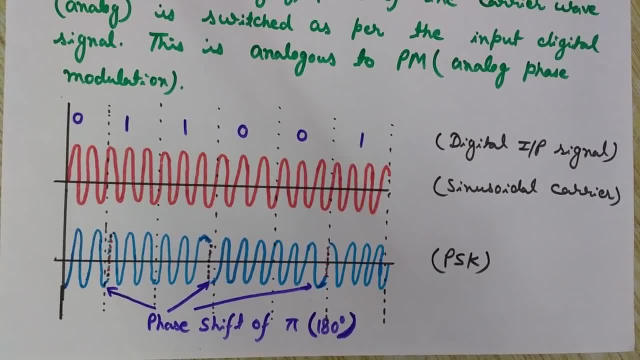 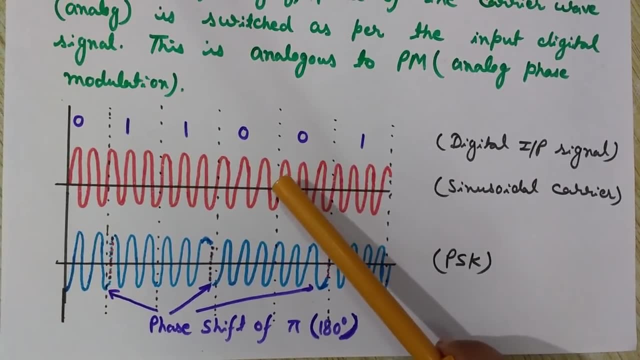 and this is the carrier wave: analog in nature. and this is the carrier wave: analog in nature, digital in nature, and now we want to perform the phase shift keying. so how to do this, since we will vary the phase of this carrier wave here according to this digital input signal. 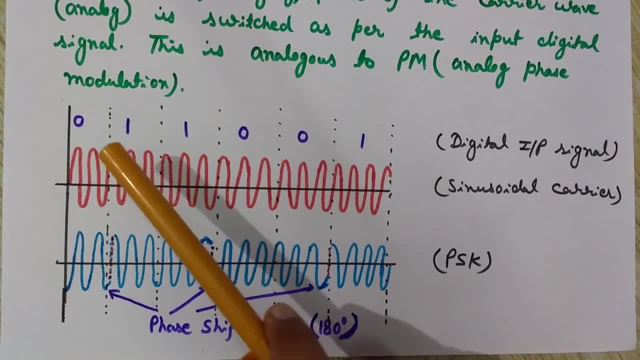 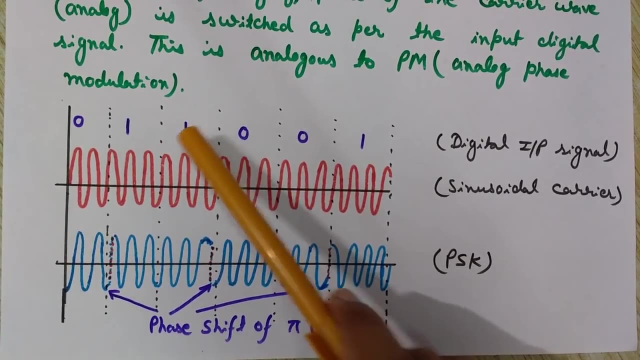 so how to do it? watch carefully. so whenever there is a change in the input signal, that is, here it is changing from 0 to 1, and here there is no change. and at this place there is a change from 1 to 0 and here it is no change, and here it has changed from 0 to 1. so whenever there 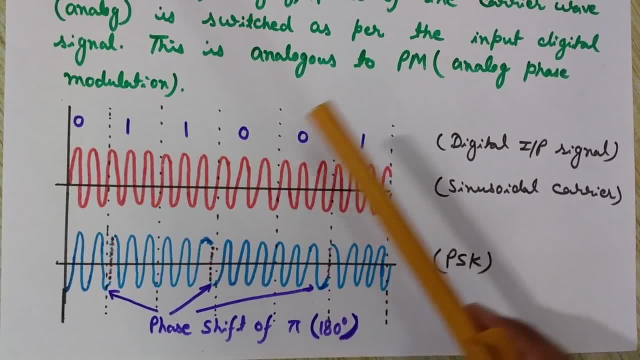 is a change from 0 to 1 or 1 to 0, a phase shift of pi that is 180 degrees, takes place in phase modulation in PSK. so let's understand it how it takes place at, since here it is 0, so there is no. 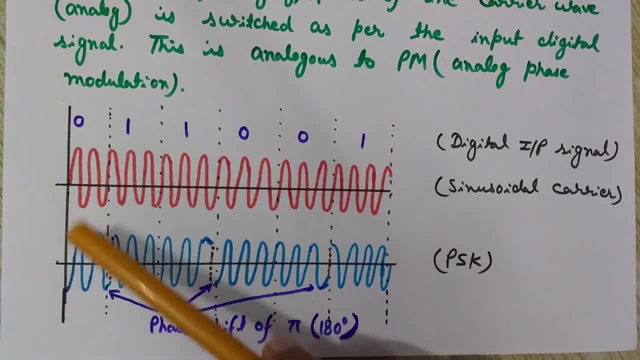 change in the wave and this carrier wave is transmitted, okay, and at this place it has been changed from 0 to 1, so phase shift has taken place here, this place- you can see here it's a. its shape was in this direction, it is was. it was going down, but it has started from upwards. 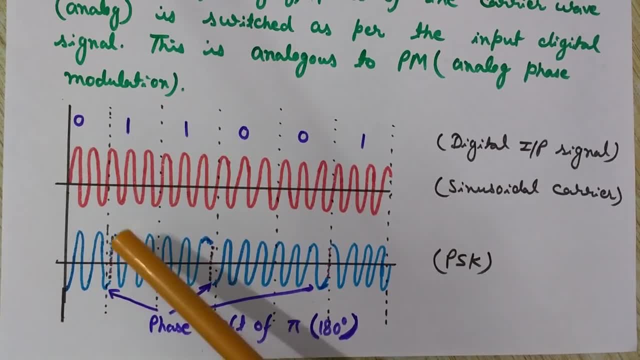 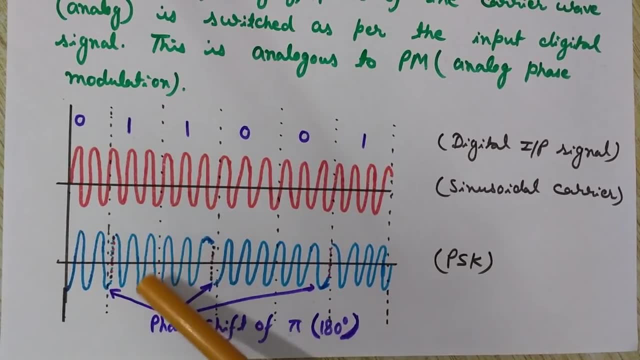 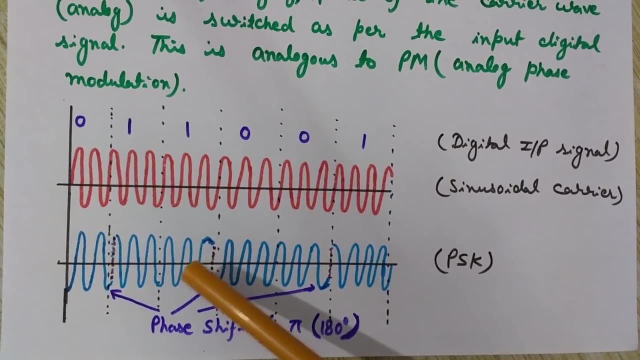 and a phase shift. this is a phase shift of pi. okay, so at this, at this place, there is no change from one to one. so it can. there is no phase shift at this place. okay, since there is no change. okay, continuous analog carrier wave is transmitted at this place, but there is a phase change from.